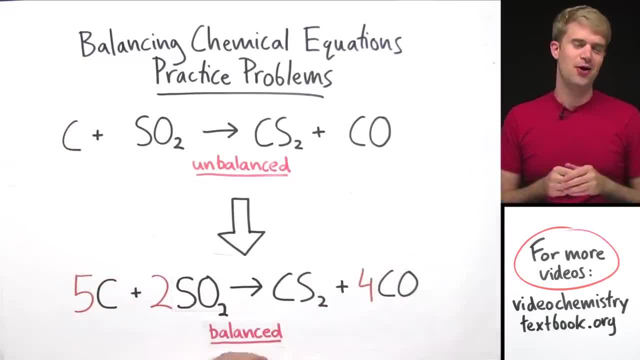 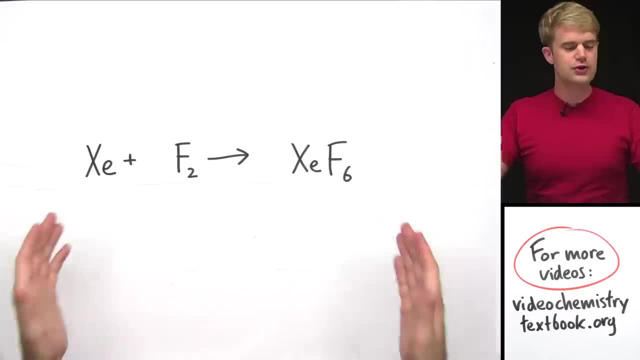 Let's do some practice problems for balancing chemical equations. We'll start off with some examples that are pretty basic and straightforward and then the problems will get more challenging as we move on. Here's our first equation. We got xenon and fluorine. We want to keep track of how. 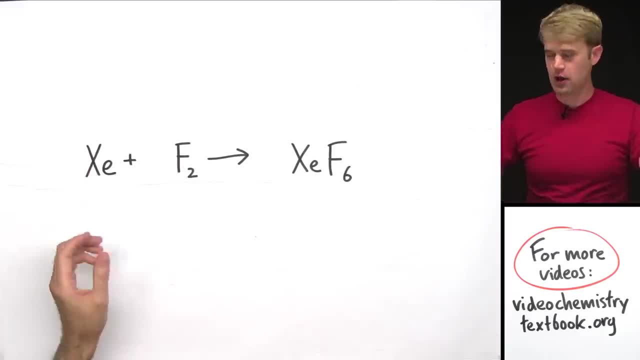 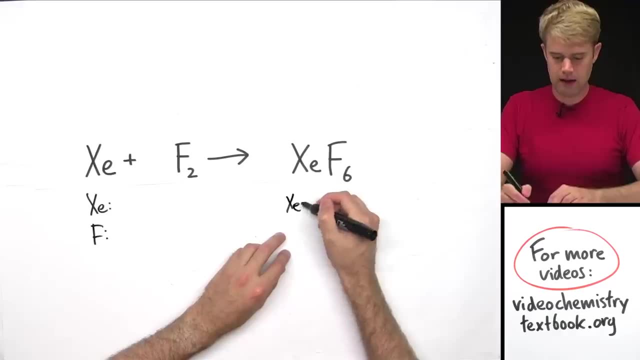 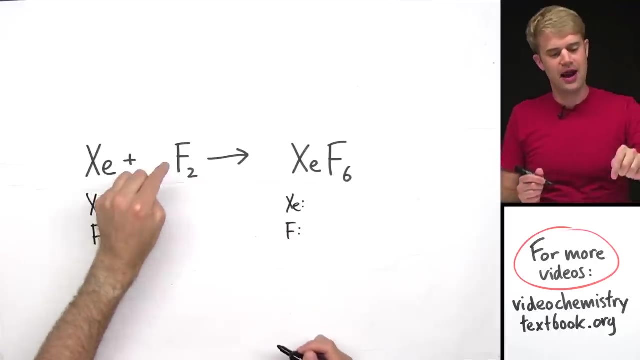 many atoms of these elements we have on both sides of the equation. so we're going to make a little chart. I got xenon and fluorine on this side and then xenon and fluorine on this side Over here. I have one xenon atom one, and then I have F2. so I got two fluorines Over here, also one xenon and 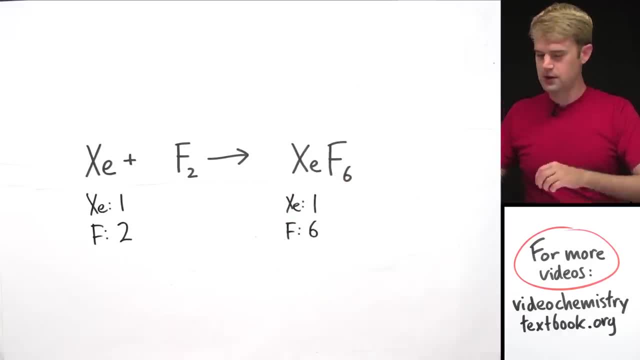 then F6, so I got six fluorines. Now take a look at these numbers. This equation isn't balanced yet because we have different numbers of the atoms for one of the elements. I've got two fluorine here, but I've got six fluorine here, so it's not balanced. In order to balance it, I've got to add numbers or coefficients. 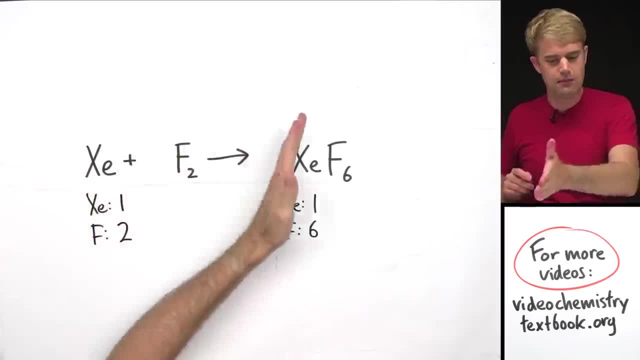 in front of one or more of these elements and compounds to change the number of atoms that I have on the different sides of the equation. Okay, here's how I'm going to do it. I got six fluorine here, but I got two fluorine here, So for this to balance, I'm going to do the following: 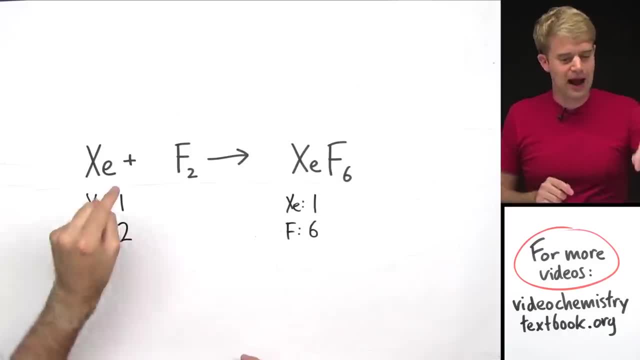 I need more fluorines on the left side. I can add a number in front of the F2 here. If I put three in front of this F2 here, we'll put it in. If I put three in front of this F2 now, I have three times two gives me six fluorine and now they balance. 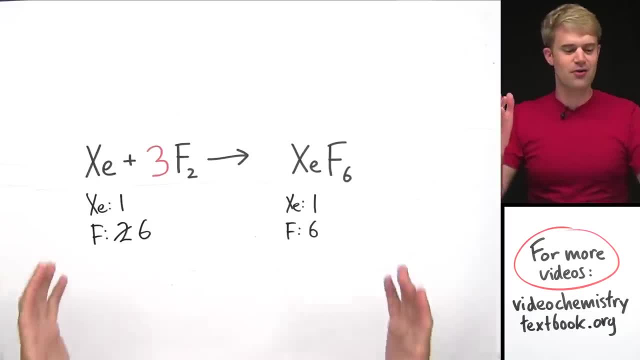 One, one for the xenons, six and six for the fluorine. So now this is a balanced equation. by adding this number, by adding this coefficient- Now, really quick. this is one very common question People often ask: wait, why did you put that three there? Couldn't you just change this two to a six? 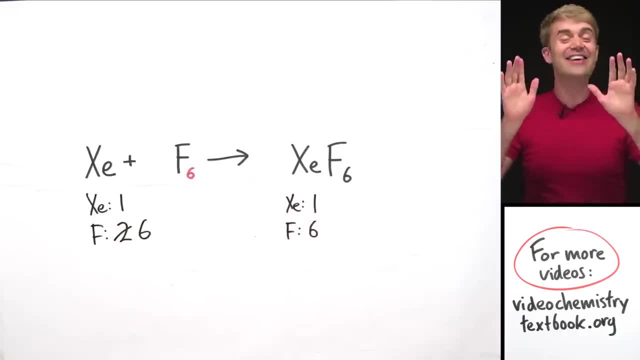 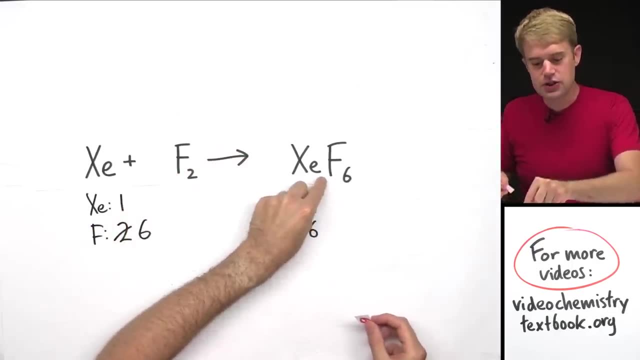 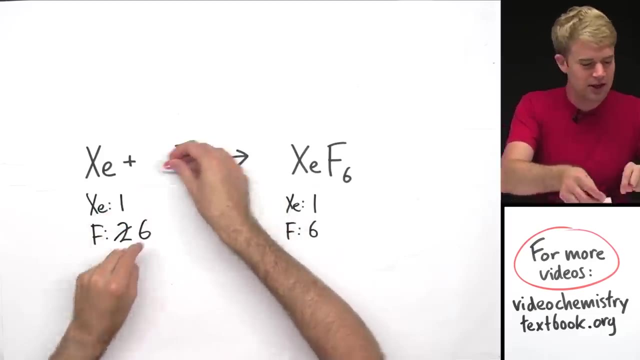 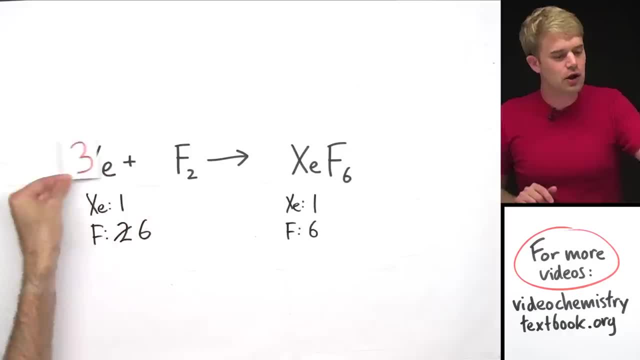 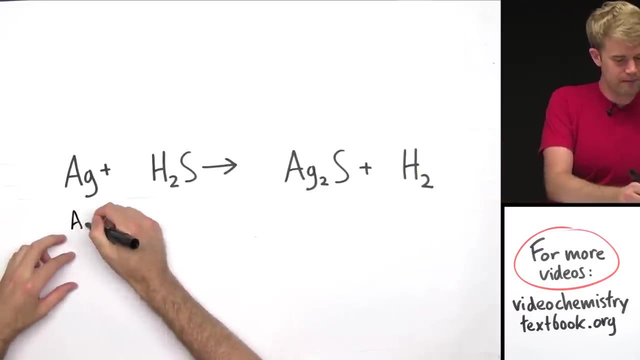 numbers in front of the elements or compounds, okay, but you can't change or add the subscripts, Okay. so that's how you balance an equation. Let's do a whole bunch more practice, Okay. so in this equation we've got three elements: silver Ag, hydrogen H and sulfur S. Obviously we've got these. 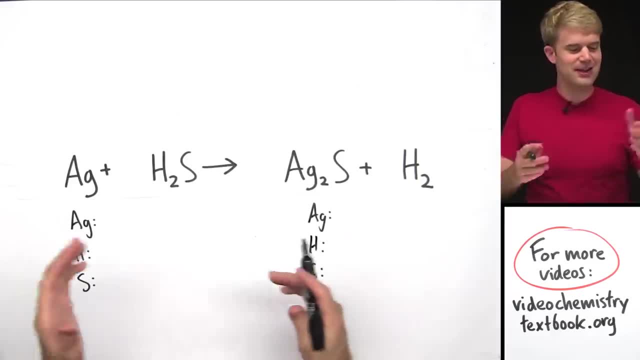 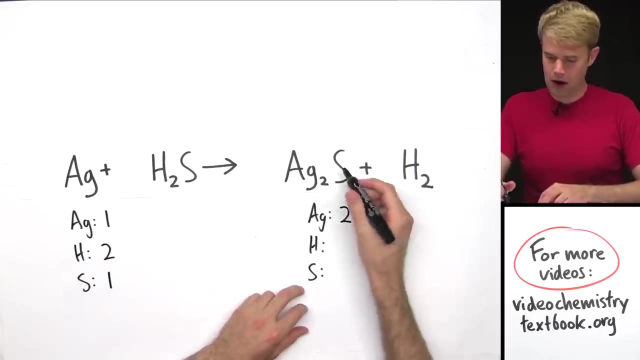 both sides of the equation. Okay. so let's see how many atoms we have of each. Over here we got one Ag. we got H2, so we got two hydrogen atoms. and we have S, so we got one sulfur atom. Over here we have Ag2, so we have two silvers here. Sulfur, we have one. and then we have H2, so we have two. 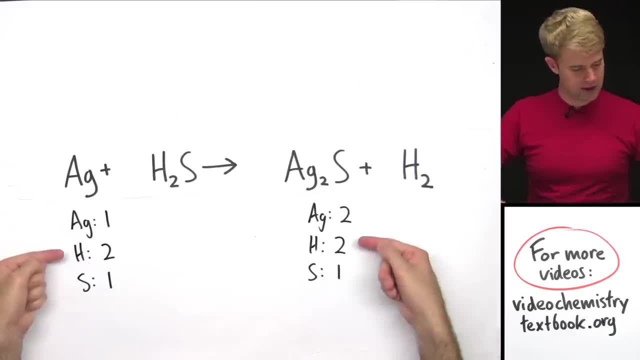 hydrogens. Okay, what balances and what doesn't? Well, the hydrogens and sulfur: both balance. but the silver we have here and one here. We can fix it by adding a number or coefficient in front of one or more of these elements and compounds. I need more silvers on this side and luckily I can just put a two. 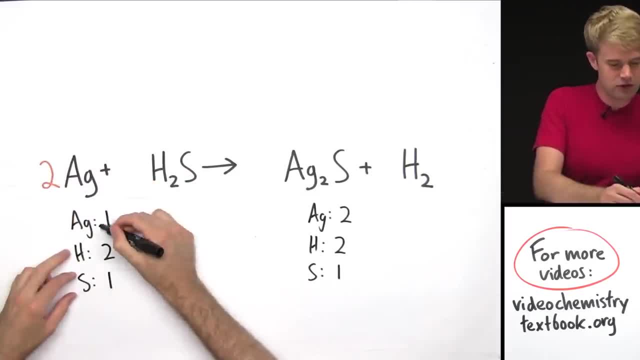 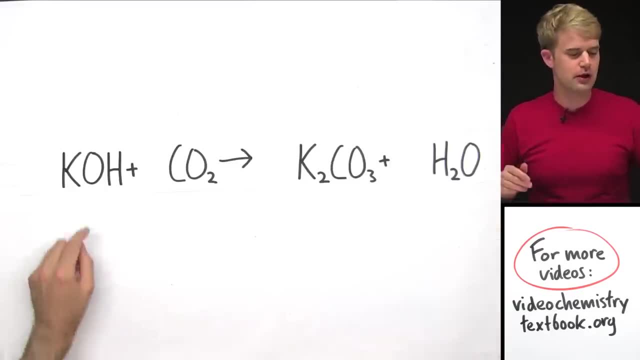 in front of this Ag. so now, instead of having one Ag, now I have two, and now I got two. two and one It balances. This equation is a little bit more challenging because we have oxygen in all the compounds here. That means we're just going to have to. 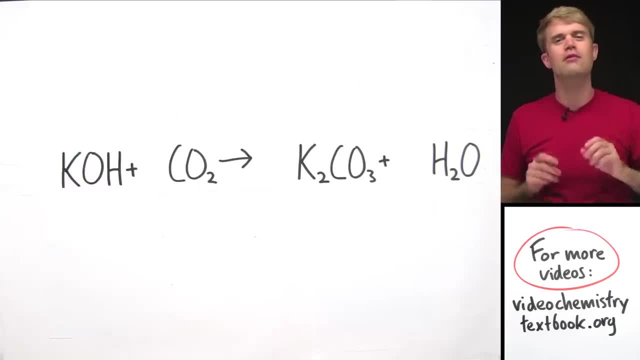 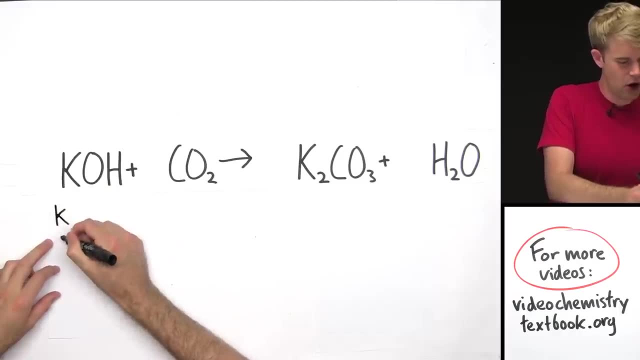 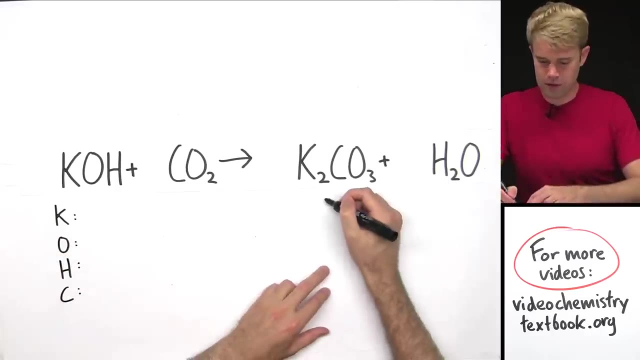 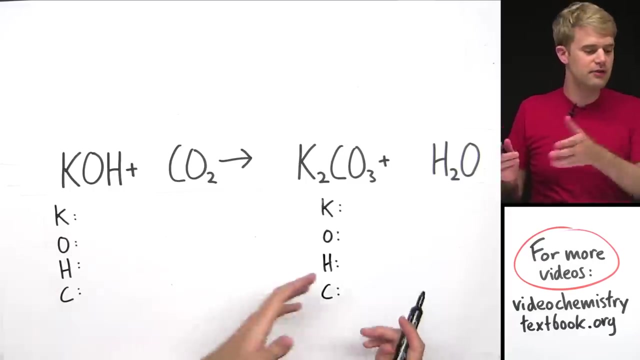 be a little bit more careful when we're adding up the number of oxygen atoms that we have. Okay, so the elements in this equation: we got K, potassium, O oxygen, H, hydrogen and C carbon, and over on this side we've got potassium, oxygen, hydrogen and carbon. Okay, how many of each? 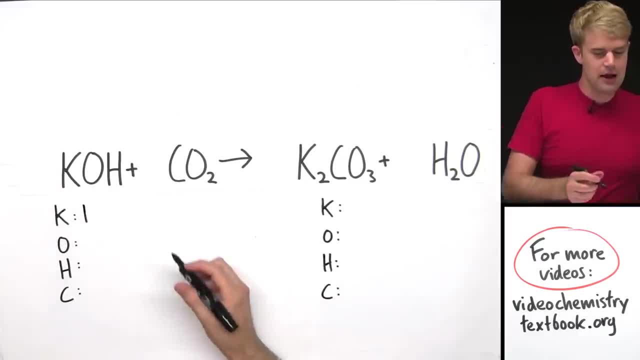 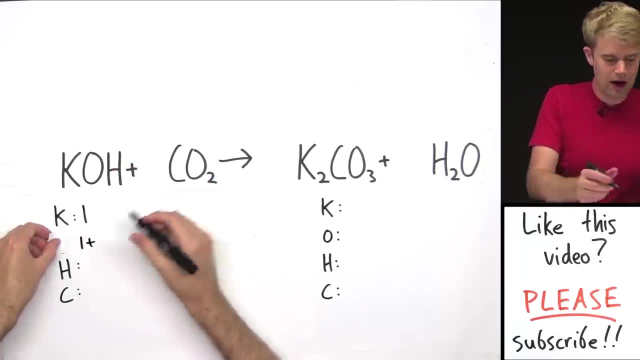 of these do we have? Okay, we got one potassium here. Now for oxygen. this is where you just got to be a little bit more careful. okay, because we have one oxygen here, but then we have two oxygens here, so one plus two, total we have three. Then hydrogen- we got one of those- and carbon- we got. 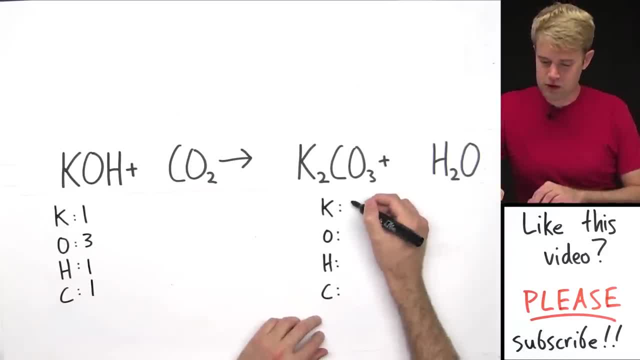 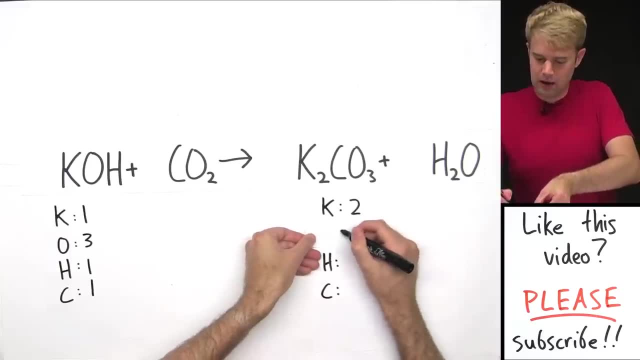 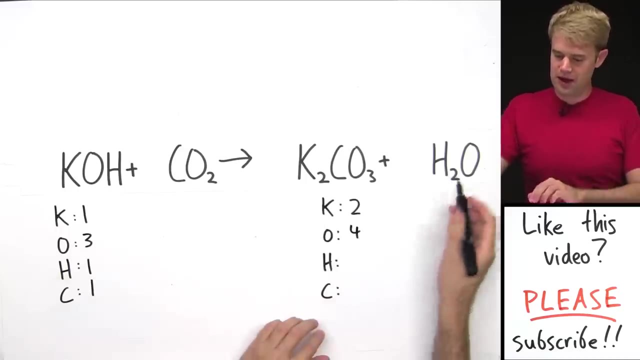 one of those Over here for potassium. we have two of these because we got K2.. Then oxygen: we have three there and we have one there. it's going to give us four total. Then we have H2. we have two hydrogens and one carbon. Okay, so what balances, what doesn't? 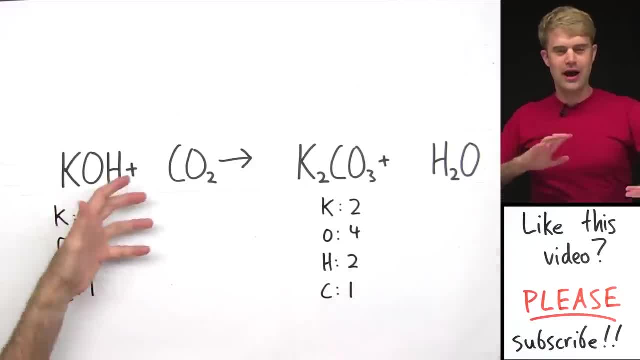 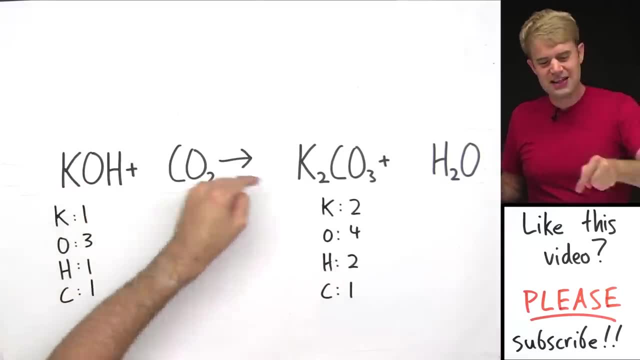 The carbons balance, but other than that, we've got to add some coefficients to change this stuff around. okay, Oxygen doesn't balance, but since oxygen is in every one of the compounds, I'm going to leave that for later. I'm going to start with potassium, because it's easier, right. 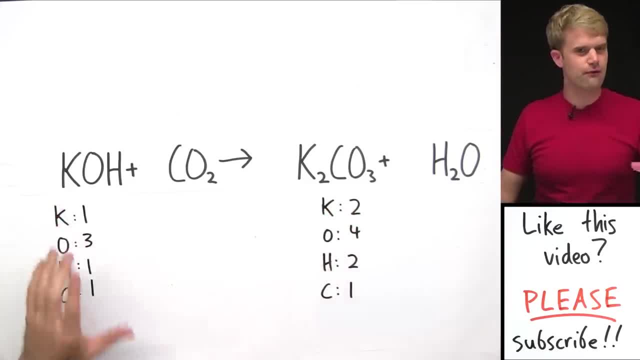 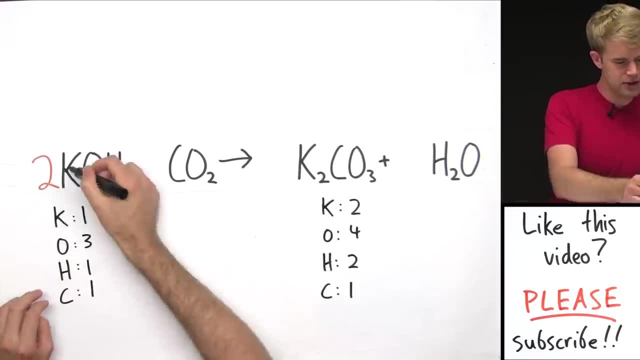 I have two potassiums here, but I've only got one here. The first thing I'm going to do is I'm going to put a two in front of this KOH and let's see what that does. okay, The first thing that's going to do is it's going to give me two instead of 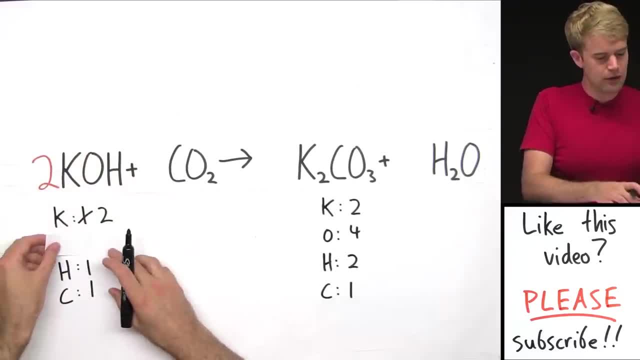 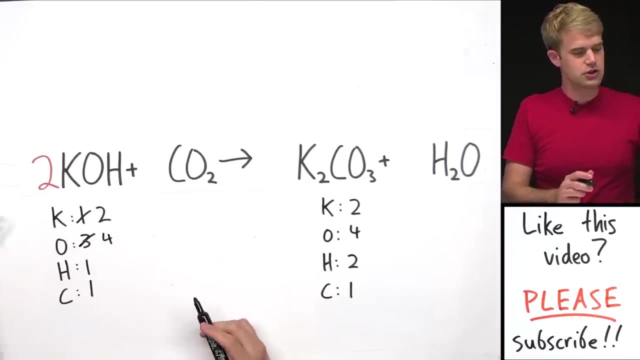 one potassium, because I have the two times K Now for oxygens. let's look at how it's going to change that. Now. I'm going to have two oxygens because two times that plus the two that I have over there in CO2- so I'm going to have two plus two- is now going to give me four, so I've got four oxygens. 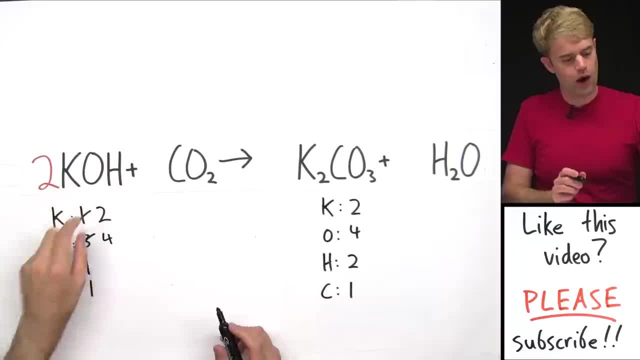 and in terms of hydrogen, now I'm going to have two times one hydrogen, so I'm gonna get two hydrogens and check it out. putting this, putting this two here, changed everything, so now I've got two, four, two, one. it all balances. Now we're going to start. 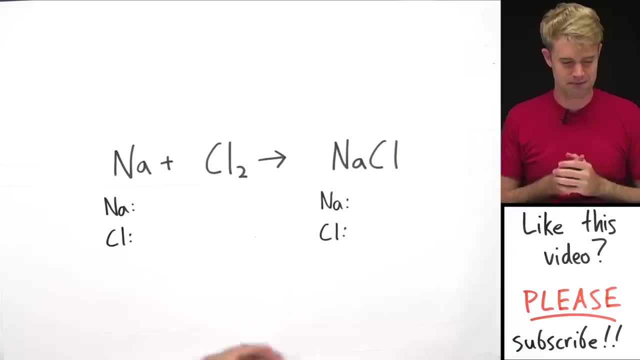 doing some equations that require more than one step to balance. okay, So this one here has sodium and chlorine. over here we got one sodium and we have Cl2. we have two chlorine atoms over here, we have two NaCl. so we have one sodium, one Na and one Cl. okay, How am I going to start? Well, I have. 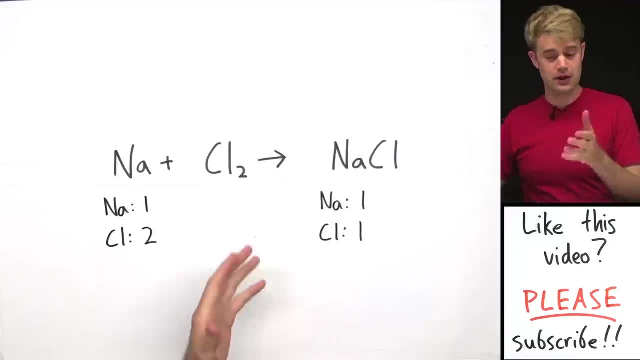 more chlorine on this side. I have two over here and I only have one here. okay, so I can start out by putting a two in front of NaCl. okay, that's going to be 2 Cl, but look what else it's going to do. okay, now I have two times Na, so I have two Na's. I also have two times Cl- okay, so I also have. 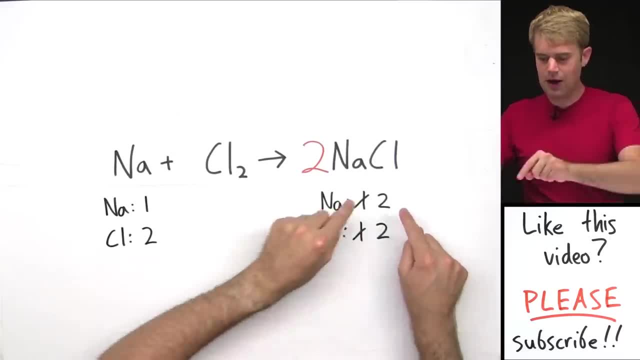 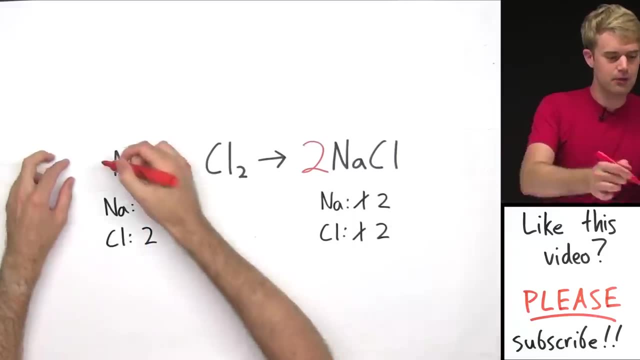 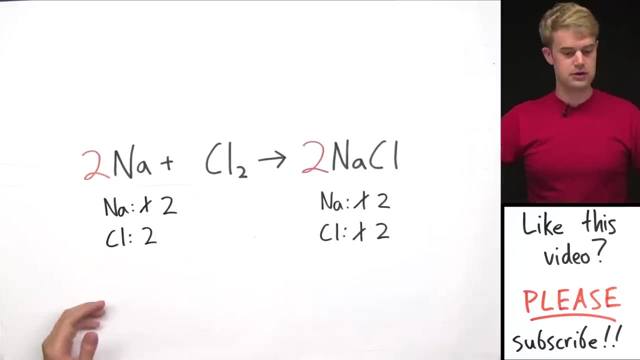 two Cl's- Cl's- balance. but now I have two Na's, two sodium, on this side. I only have one on this side. so now, to balance this out, I'm going to put a two in front of this Na here and now I have two of these. 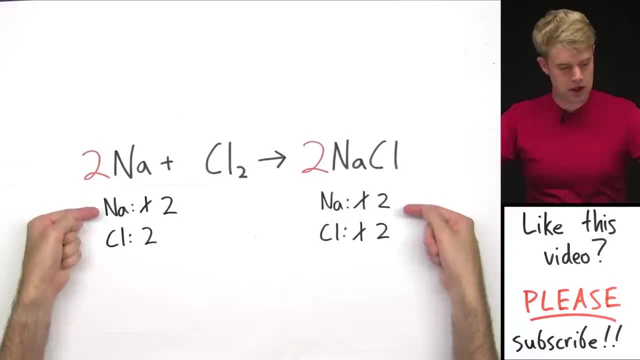 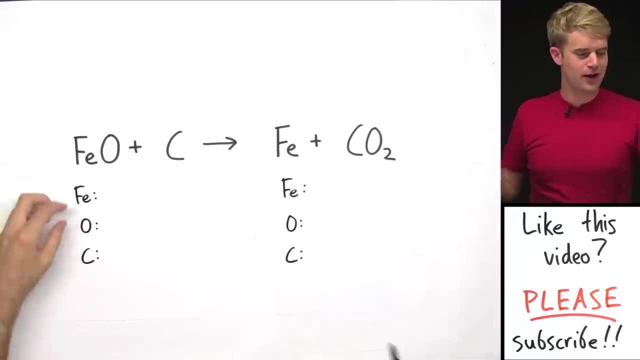 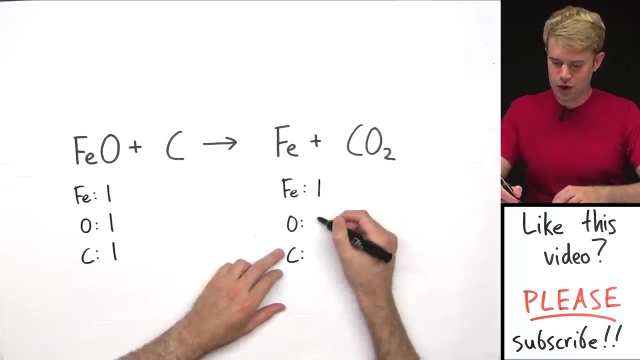 so now, on both sides of the equation, I have two sodiums and two chlorines. the equation balances: okay, iron, oxygen and carbon. over here I have one iron, one oxygen and one chlorine. here I have one iron, two oxygens and one carbon. okay, how am I going to balance this? the first: 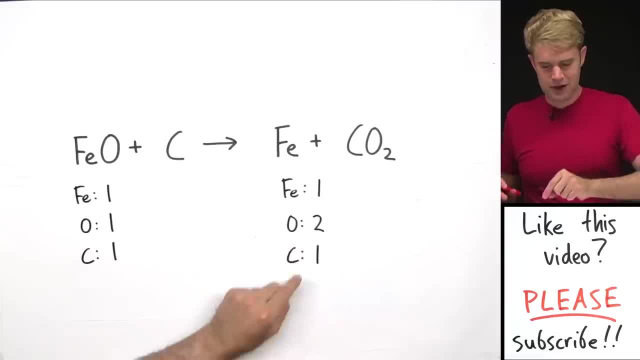 thing I'm going to do is I'm going to balance these oxygens. okay, so I have two over here and I have one here. I'm going to change that by putting a two in front of the FeO. okay, so that's going to give me two oxygens, but it's also now going to multiply this Fe by two. so now I'm going. 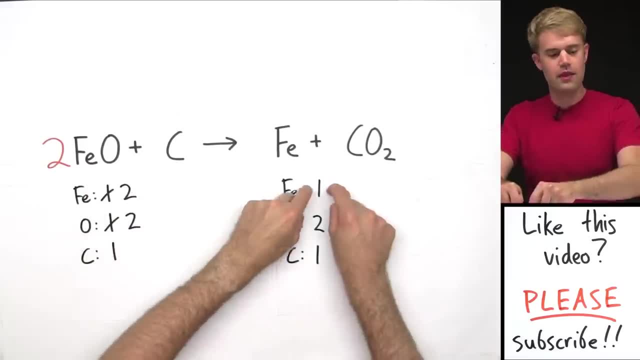 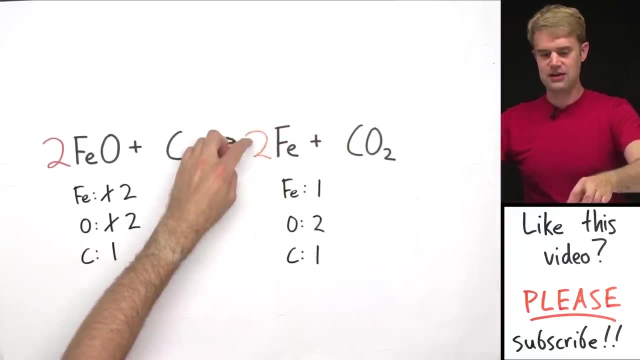 to put a Fe. okay. so now I've got two Fe here and one there. so now these don't balance. so the next thing I'm going to do is I'm going to put a two in front of this Fe there. so now, instead of having one, I have two of them. now I have two, two, one. it balances okay. let's look what we have here. we have 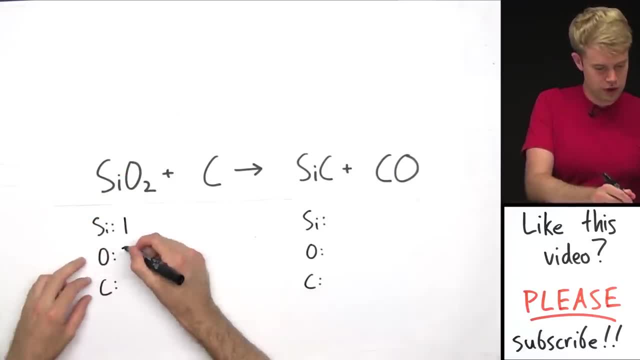 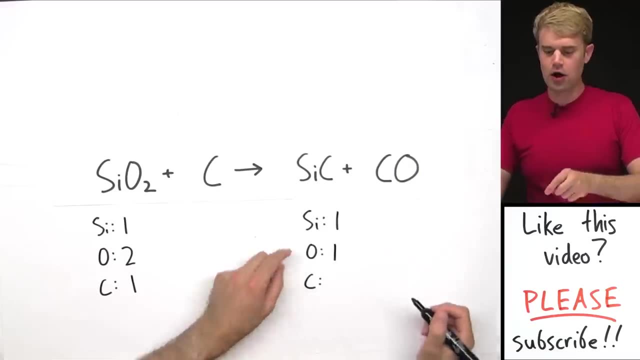 silicon. on this side we have one of them O2, two oxygen and one carbon. over here, we have one silicon, we have one, and carbon we have one plus one, so we have two. okay, so what doesn't balance? well, the carbons don't balance and the oxygens don't balance. I'm going to leave the carbon alone. 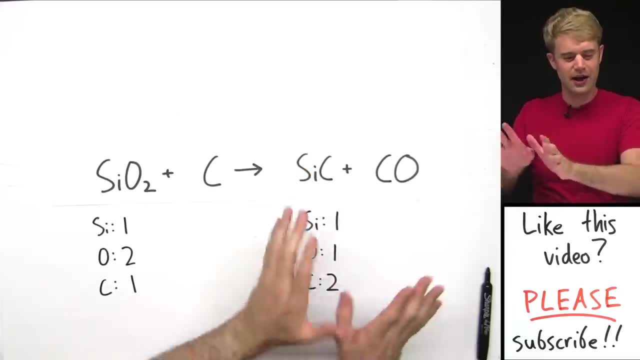 for now, because it's in both of these compounds, so I kind of don't want to mess with it right now, but I could. I'm just going to start out with the oxygen. okay, I have two oxygens on this side and I have one oxygen on this side, so I'm going to multiply the CO. 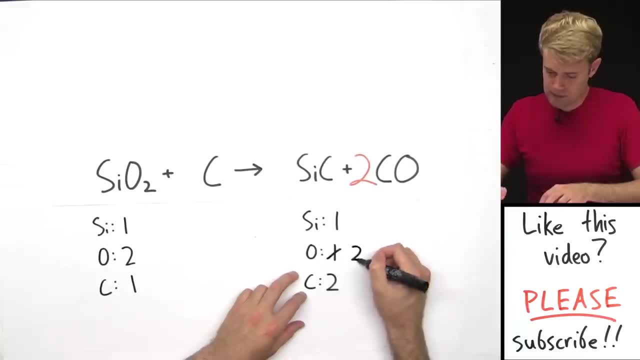 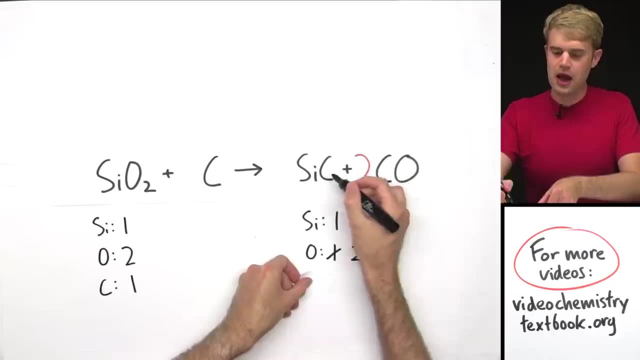 by two, so that can give me two oxygens. but now it's also going to do something else, right, because we're also multiplying this C by that two. so that means now for the total carbons I'm going to have the one from there plus now the two from there, and that's going to give me a total now of 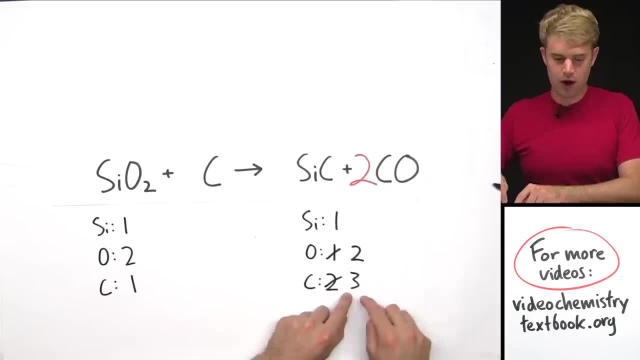 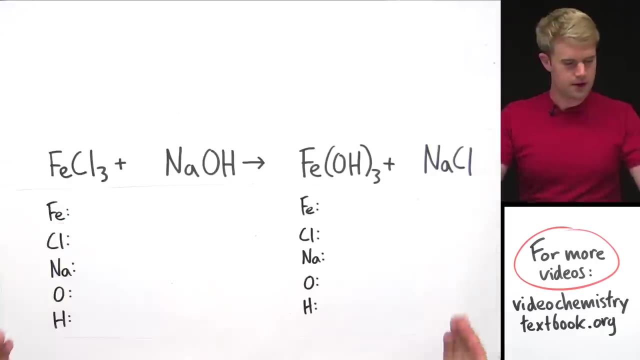 three. okay, so now I have three carbons here. I've got one carbon here, so I'm going to put a three in front of this carbon. that's the only carbon on this side. so now I have three times. one is three, one, two and three and they balance. this equation has five different elements in it. 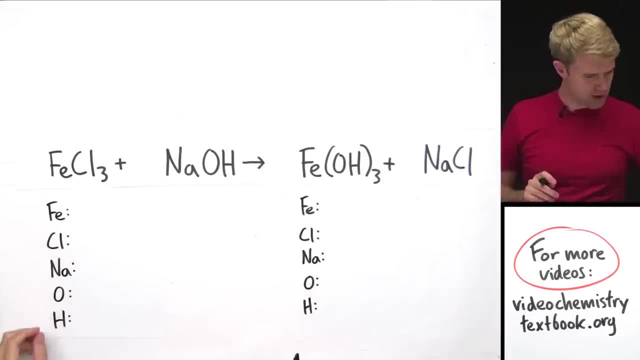 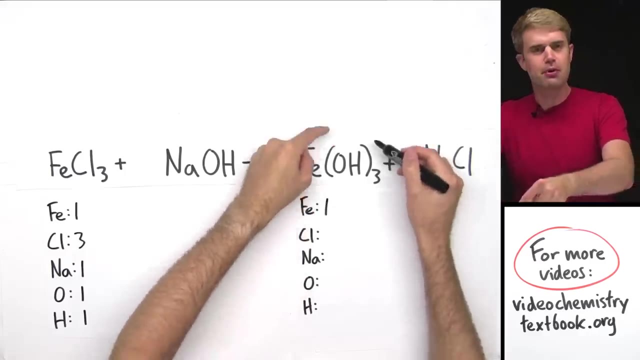 and it also has these parentheses. so we'll talk about these in a minute. first the number of atoms: iron, fe- we have one here- cl3, na1, o and h- we have one of those, okay. now fe- over here, we have one, and then we got the parentheses, okay. so the parentheses mean that everything inside here. 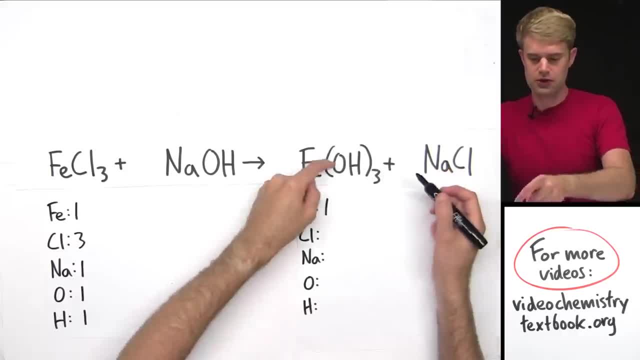 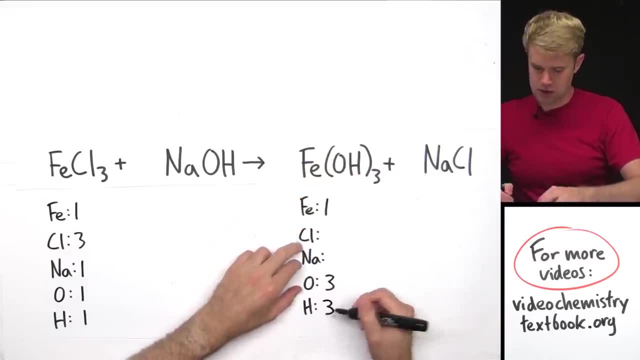 is multiplied by the number of atoms, and then we have the parentheses. okay, so the parentheses mean that everything inside here is multiplied by three. okay, so we have o times three, which means we have three o's, and we have h times three, so that's three h's. and then we have na and cl, so one each of those. 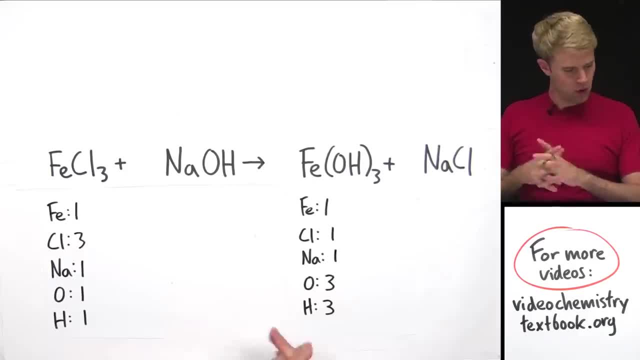 okay. so where are we going to start with this? well, I have- uh, I have- an imbalance in my oxygens here, so I might as well just start there, okay, so three here, one over here. so I'm going to put a three in front of na ho h. okay, so that is going to multiply all the stuff by three and I have three. 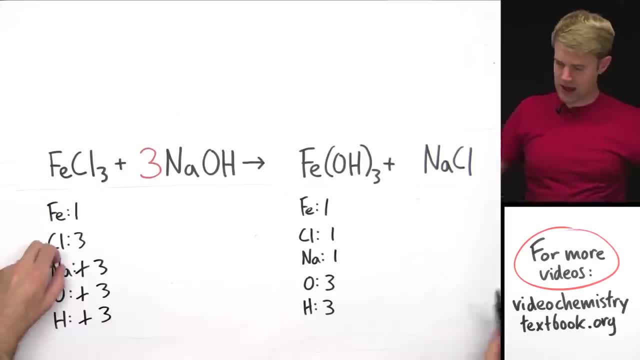 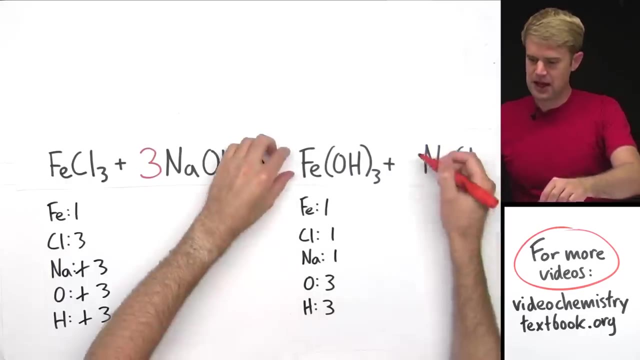 na, three o and three h. okay, what did that do for me? well, that balanced the oxygens and hydrogens, but now the sodium, the na. I have three on this side. I only have one on this side. okay, so I can fix that by multiplying this na, cl by 3 here. okay, so that's going to give me 3na and it's also going to be. 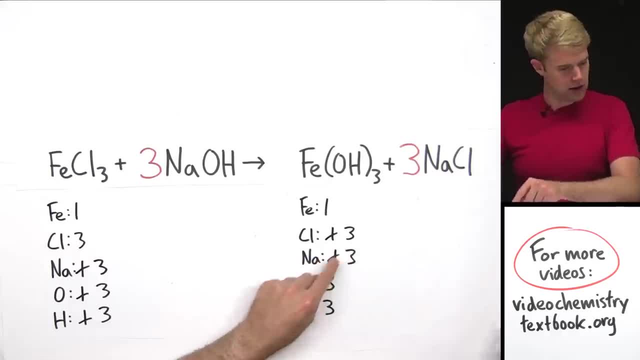 times a Cl. so now I have three Cl and check it out, that fixed it. I have three Cl over here but I got three Cl there. great. so one, three, three, three, three. it balances. we got some more parentheses here. let's take a look at this equation. 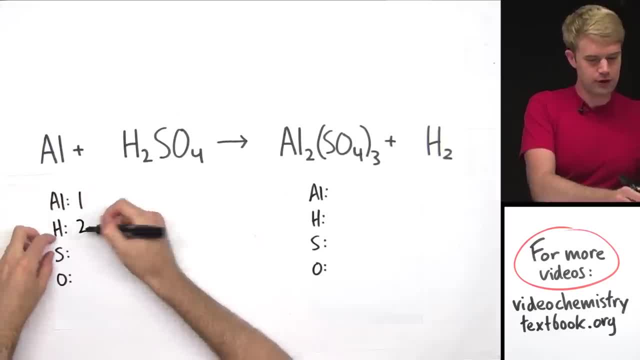 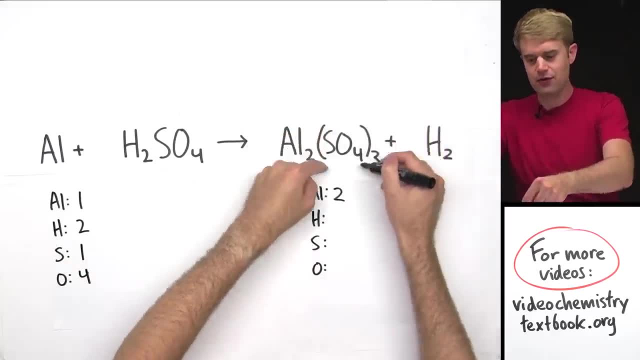 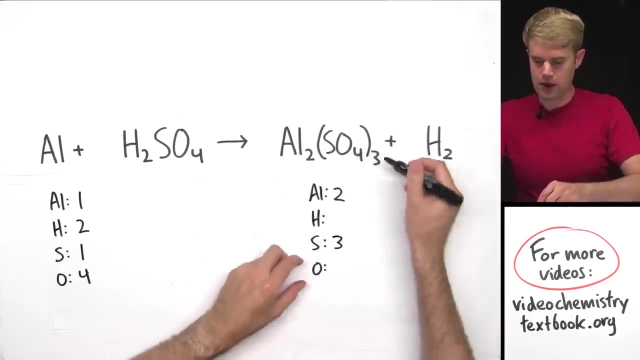 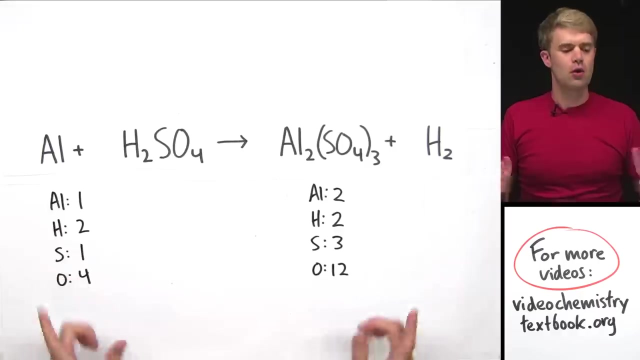 okay, I have one aluminum, two hydrogens, one sulfur and four oxygens. then over here I have two aluminums. everything in here is multiplied by three, so that means that I have three sulfurs and I have four times three, which is twelve oxygens. and then I have two hydrogens. okay, what am I going to do first? well, 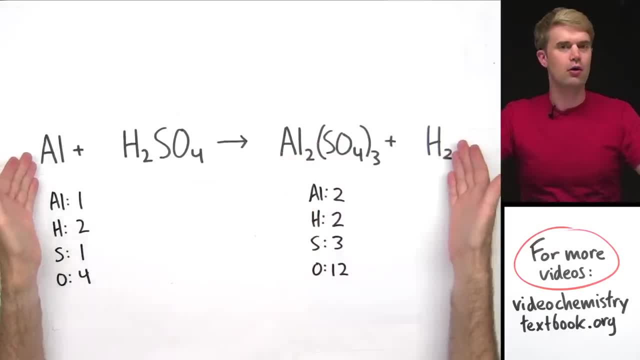 take a look at this. we have aluminum and we have hydrogen on their own, so I'm going to save them for last. I don't want to balance them right now, because we can use these at the end to straighten out some of these details. so let's look. 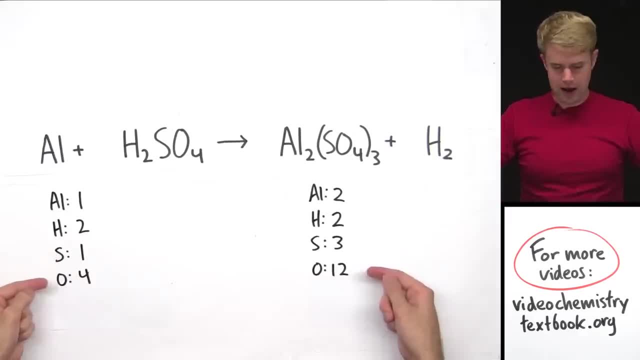 right now it's sulfur and oxygen. I can fix both the sulfur and the oxygen in the balance them by multiplying these by three. right, I have three sulfurs and 12 oxygens. so if I just multiply these by three, I can get them to balance. so I've 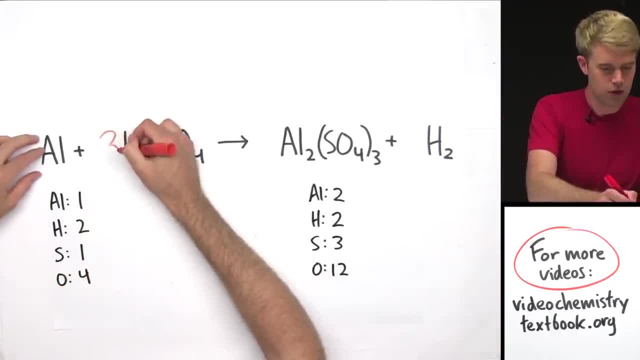 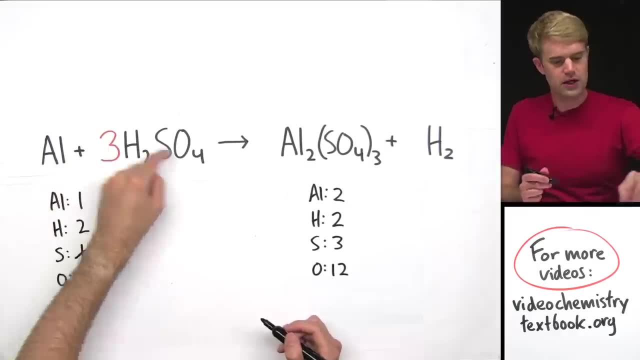 got sulfur and oxygen there, so I'm going to start by putting a three in front of that, okay. that's then going to give me three sulfurs and three times four, 12 oxygens, and it's also going to give me some more hydrogens, okay. so now I got six hydrogens, okay. so we can see that I've 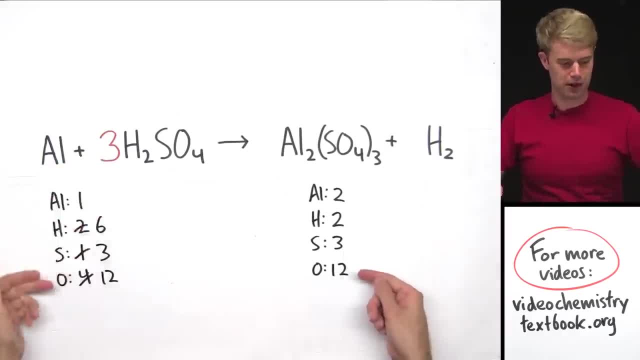 We got the sulfur and the oxygen to balance now just by multiplying by 3.. Now my hydrogen, my hydrogen, doesn't balance. I have 6 on this side, 2 on this side, So I can fix that by multiplying the hydrogen by 3.. 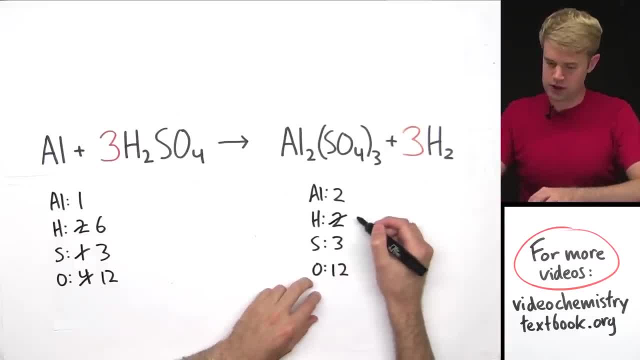 Now I have 3 times 2 on this side, which is going to give me 6.. And then take a look at the aluminum. I have 2 on this side, 1 on this side, but I can fix that by multiplying by 2 over here. 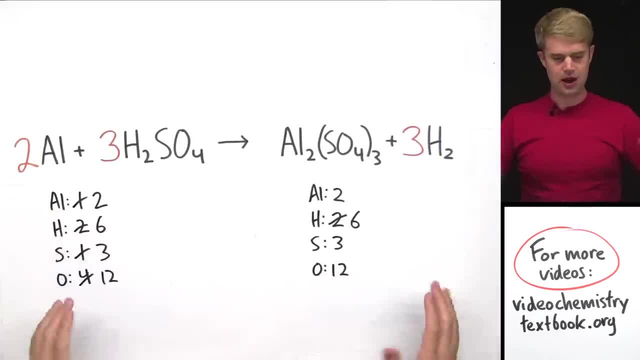 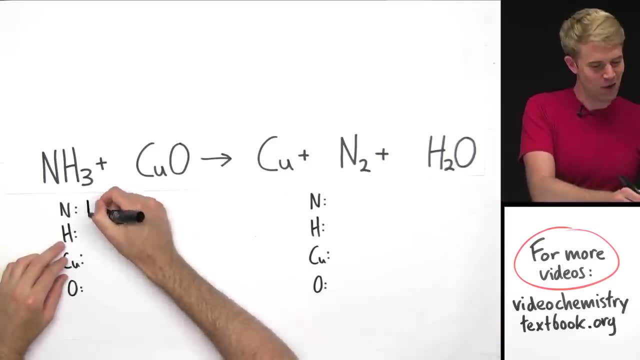 and then I get those to balance and everything is good. You may have noticed these are getting a little bit more complex. it takes more and more steps to balance them. Okay, so for this, we have 1 nitrogen, we have 3 hydrogens, we have 1 Cu, which is copper. 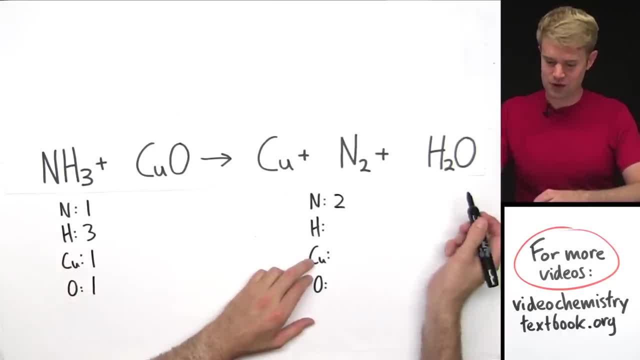 and we have 1 oxygen Over here. we have 2 nitrogens, 2 hydrogens, 1 copper and 1 oxygen. Okay, where am I going to begin with this? Well, copper and nitrogen Hydrogens are on their own here, so I'm going to leave them to last.